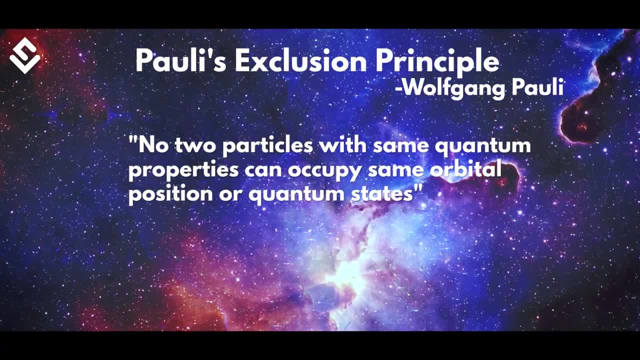 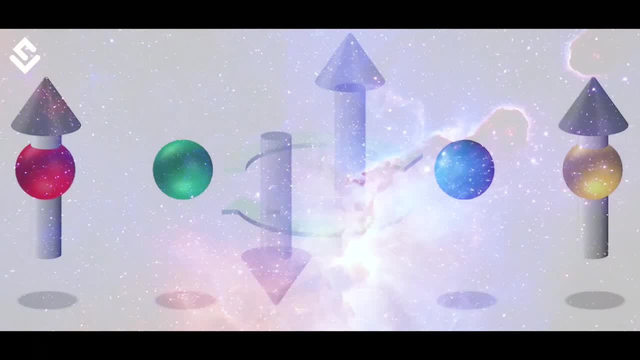 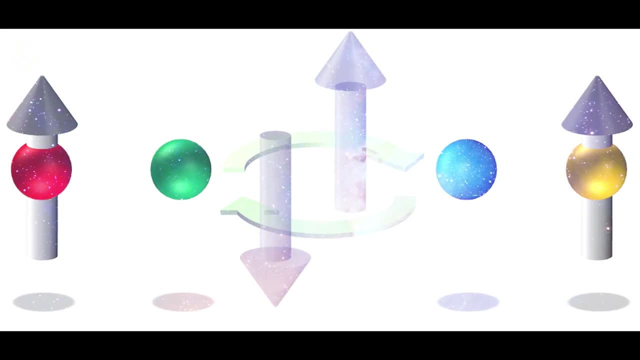 can occupy same orbital position or quantum states. So if one electron has spin clockwise, then other must have its spin anti-clockwise. The spin is a quantum property of particles that is related to intrinsic angular momentum of the particle rather than actual spinning. 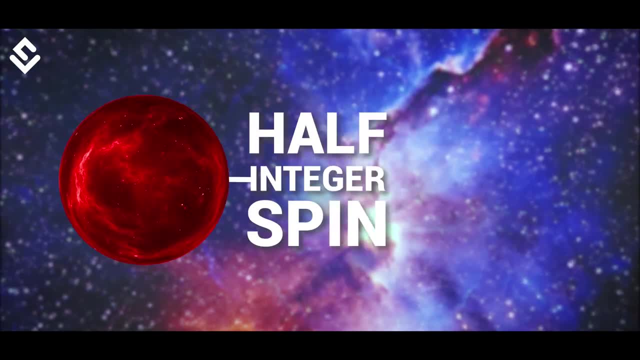 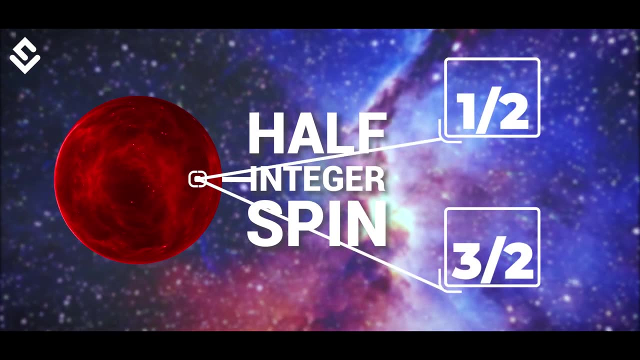 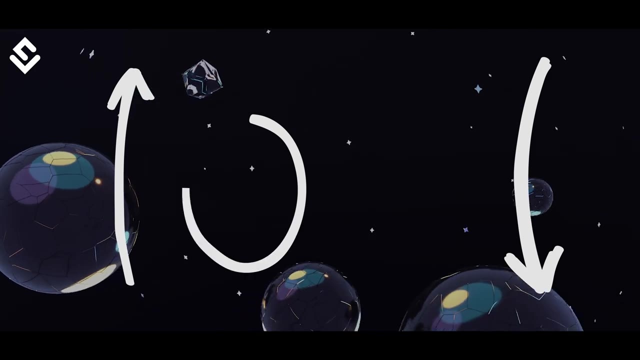 as the name suggests, Fermions are the particle with half integer spin, which means mathematically their spin states are represented by one, half, three halves, etc. Also, spin states has particular orientation, such as upward, downward or clockwise and anti-clockwise. An electron has spin value. 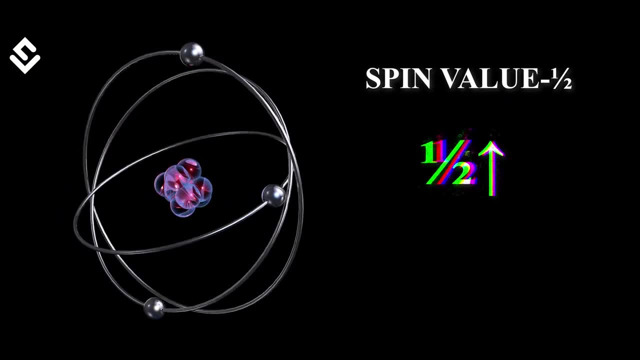 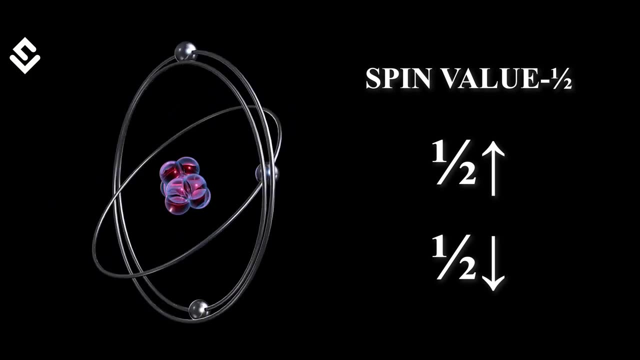 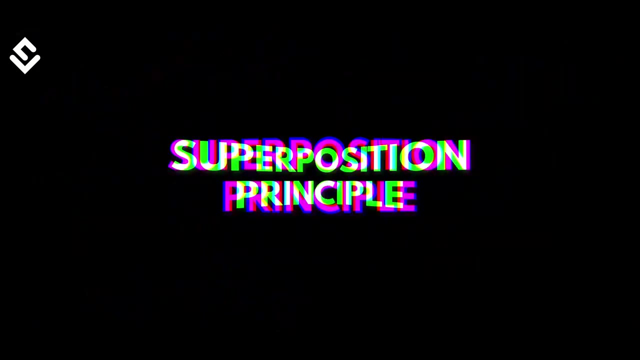 of one half, and thus it may exists in two states that are one half up and one half down, Since quantum particles shows their states only in probabilities and thus there are always certain probabilities that both these states can co-exist simultaneously. This property is called the superposition principle, The 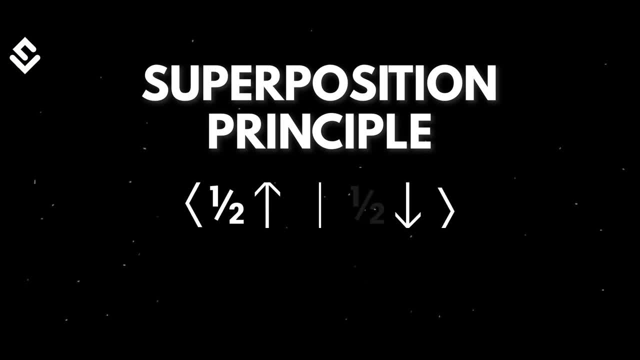 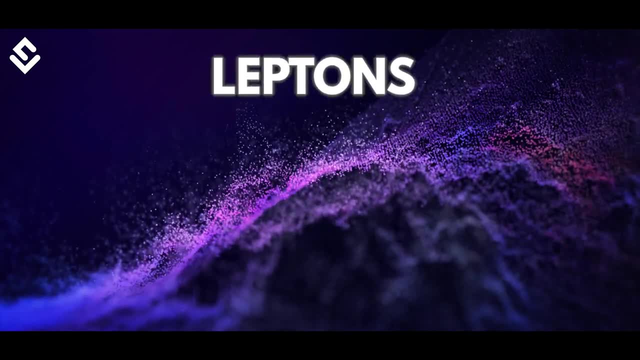 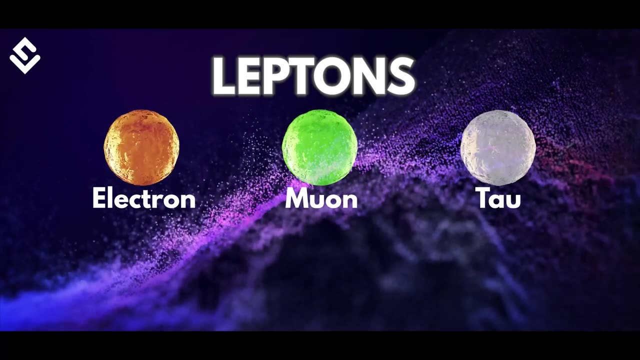 arrangement can be shown mathematically using bracket notations. Fermions are of two types: Leptons and Hadrons. Leptons are elementary particles and they consist of six particles: Electron, muon, tau and 3 neutrino components. 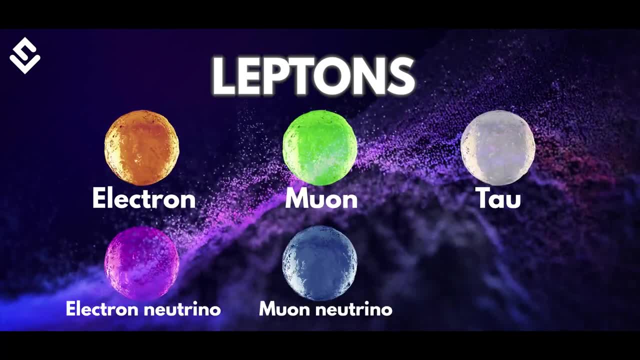 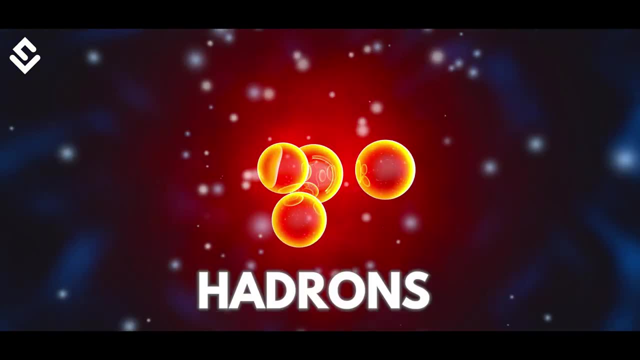 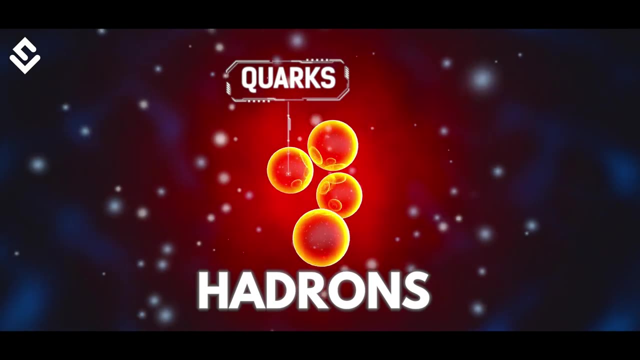 of these particles, particles electron neutrino, muon neutrino and tau neutrino. They all have spin value of one half. Hadrons are composite particles that are composed of two or more constituent particles. These constituents are called quarks. 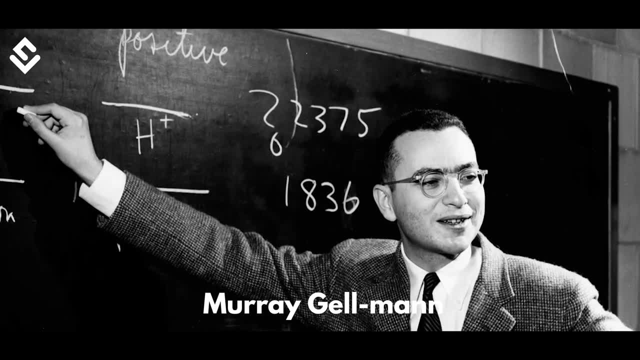 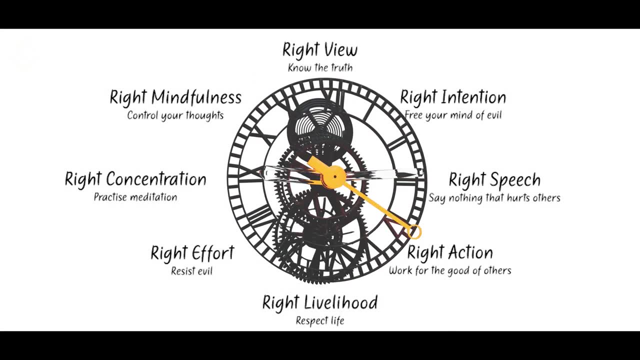 The term quark was coined by Murray Gell-Mann in 1960s. during the formulation of quantum chromodynamics, Gell-Mann proposed a new method inspired by Buddha's Eightfold Path to organize all the different sets of new particles being discovered in 50s and 60s. 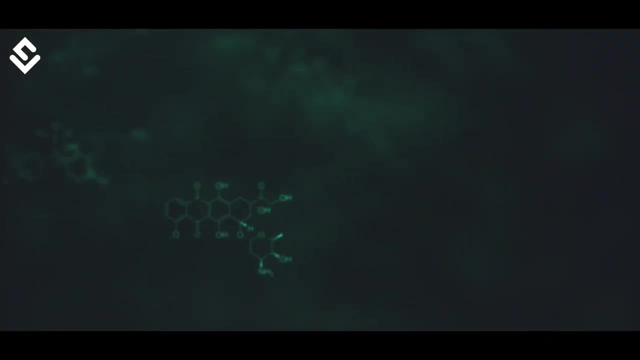 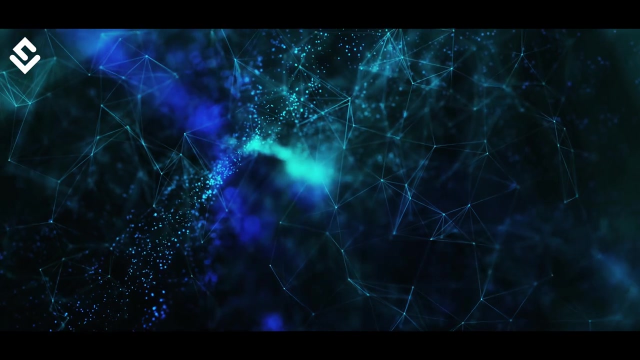 He arranged the particles with respect to two quantum properties shown as isospin and hypercharge, and proposed the relation between them. He found out that all these heavy particles are behaving like composite particles, forming various series like octet, doublet and triplet. Components of these particles were named quarks, and they are of six types: Up quark, down quark, top quark, bottom quark, charm quark and strange quark. Why were they named like this is a different mystery altogether, but let's focus on Hadrons. 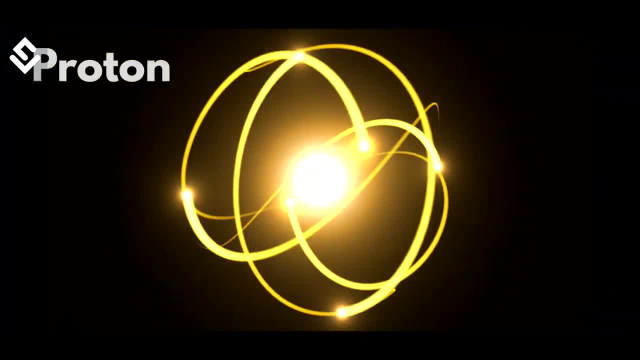 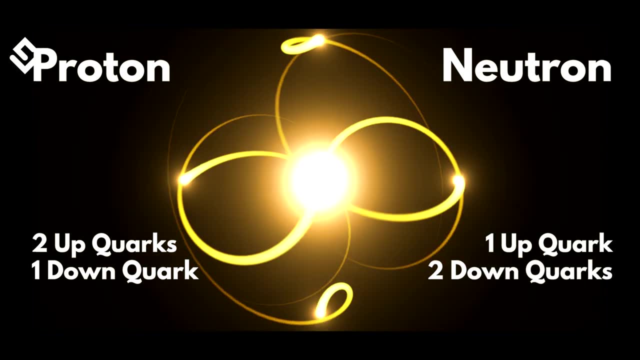 Protons and neutrons are two examples of hadrons. A proton is composed of two up quarks and one down quark, while a neutron is composed of one up quark and two down quarks. Each quark has charge values in terms of one third and two thirds. All upper family quarks, such as up top and charm, have two thirds charge and the lower family quarks is down bottom and strange- have one third. All upper family quarks, such as up top and charm, have two thirds charge and the lower. 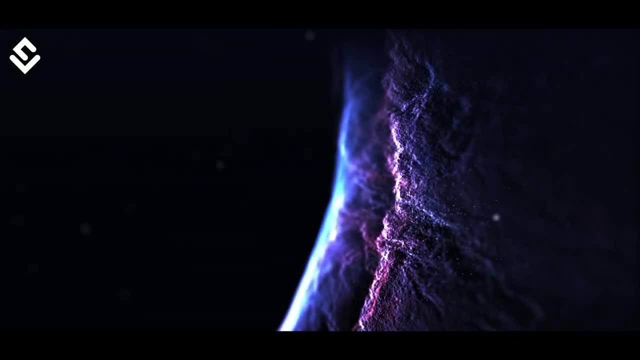 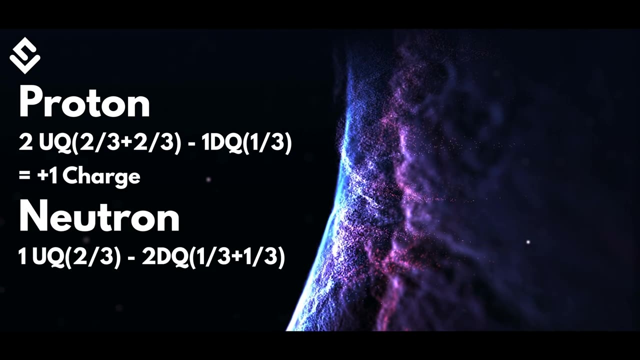 family quarks is down bottom and, strange, have one third, 1. 3rd charge: Let's count: Proton has composition of 2 up quarks and 1 down quark, so total charge will be plus 1, while the neutron has sequence of 1 up quark and 2 down quarks, so total charge 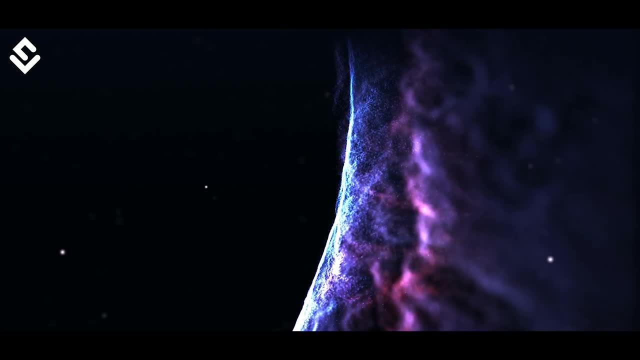 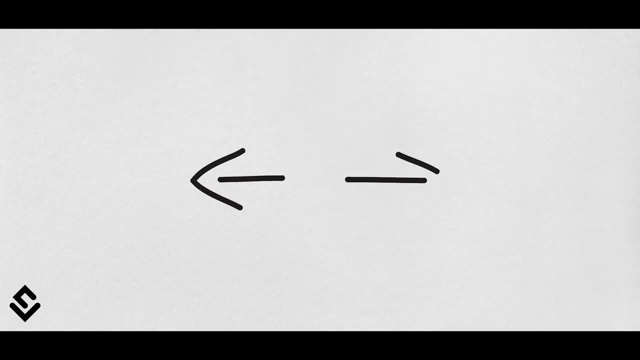 will be 0. I think that's simple and precise. Now let's move to boson part. Bosons are particles responsible for production of forces. There are 4 fundamental forces in nature, and they are: electromagnetic force, strong nuclear force, weak nuclear force and gravitational force. 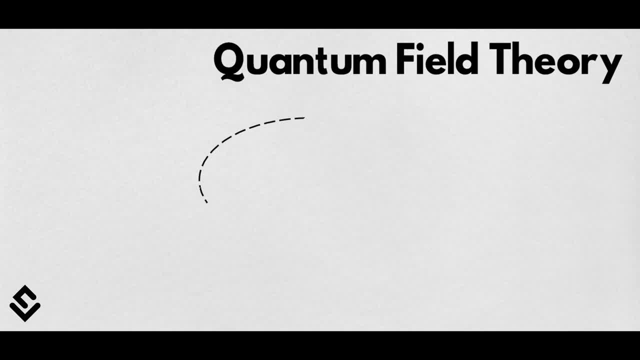 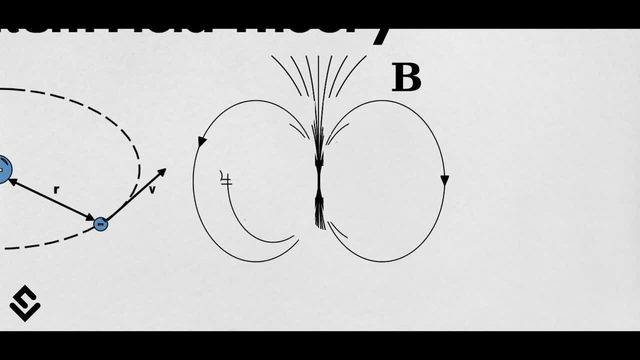 According to quantum field theory, a moving charge creates a changing field in its vicinity and which travels throughout the space and time. Any object that passes through this generated field will feel the effect of force. This field is the distortion of the space-time and the quantization of the. 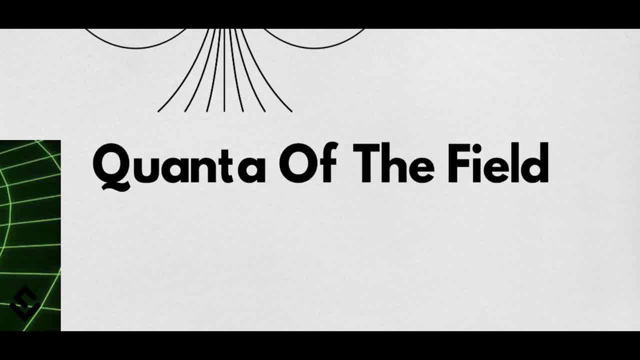 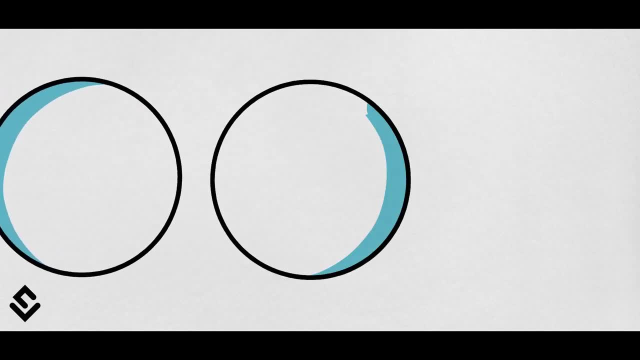 field is by particle, known as the quanta of the field. Thus, electromagnetic field is propagated through the quanta we know as the quantum field. The quantum field is the quantum field of the photon. We can say that two electrons coming toward each field repulsive force. This is because 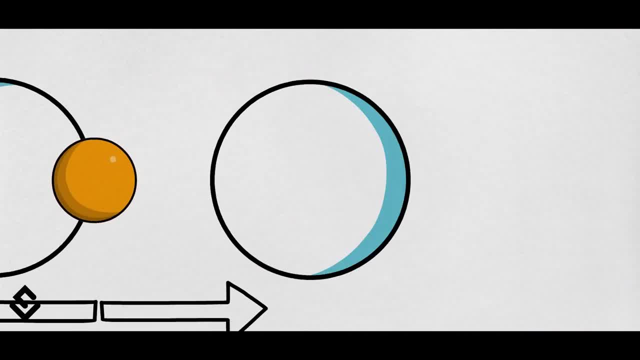 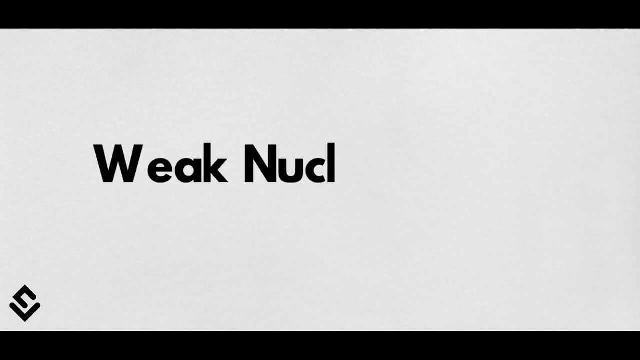 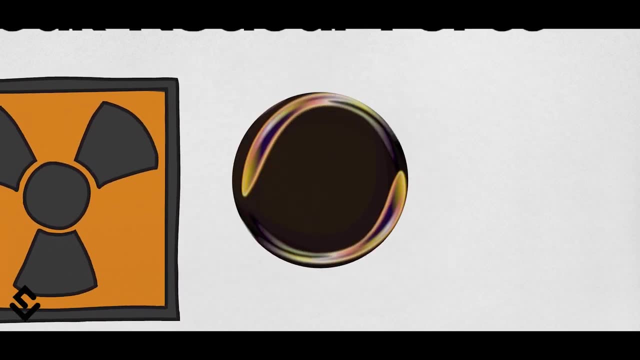 an electron emits a photon that hits the other electron and pushes it away, and this repulsion is the repulsive electromagnetic force that electron experience. Weak nuclear force is responsible for radioactive decay happening in the material. A neutron which decays into proton can be interpreted as neutron emitting a weak particle and that weak particle again gets. 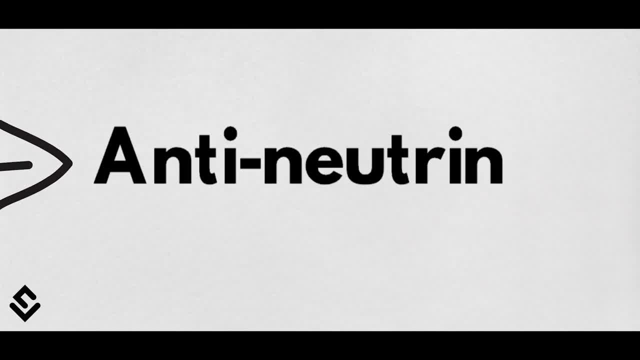 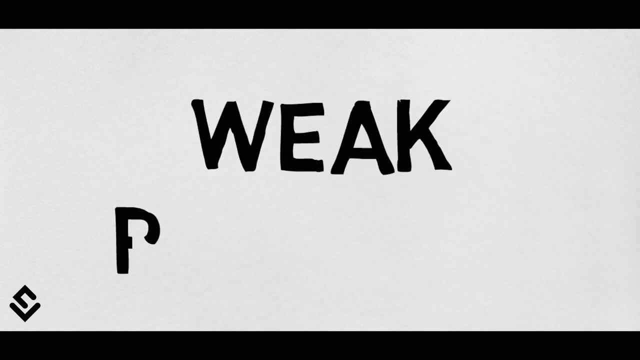 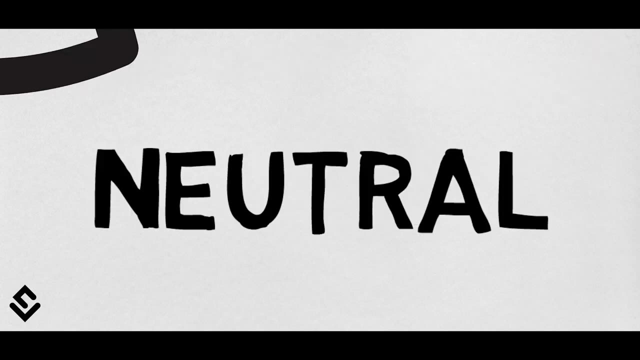 divided into electron and anti-neutrino, Thus neutron. shedding an electron makes it positive, that is a proton. From here we can understand that there must be a weak particle for all three types of interactions: positive, negative and neutral. So there are three weak particles and they are: